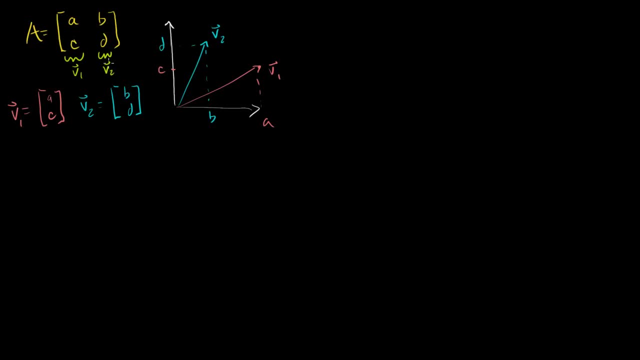 And what I mean by that is: imagine that these two guys are position vectors that are specifying points on a parallelogram, And then, of course, the 0, or not, of course, but the origin is also another point on the parallelogram. 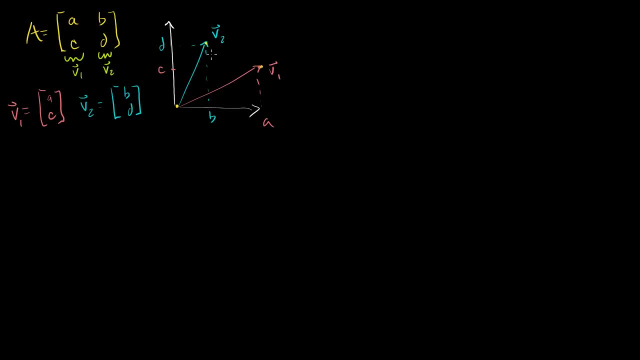 So what will be the last point on the parallelogram? Well, you can imagine a parallelogram. we already have two sides of it, So the other two sides have to be parallel. So one side will look like that. It's parallel to v1, the way I've drawn it. 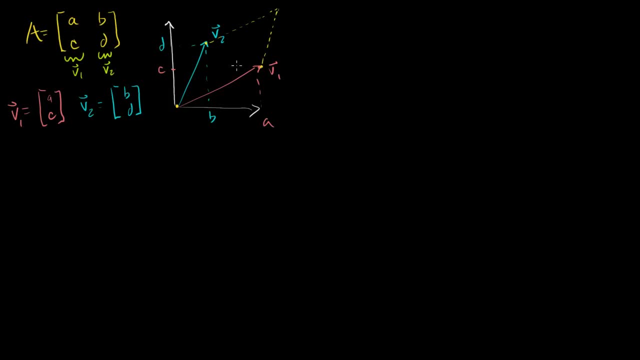 And then the other side will look like this: That's our parallelogram. And then the other side will look like this: That's our parallelogram, The parallelogram generated by v2 and v1.. What we're going to concern ourselves with specifically is 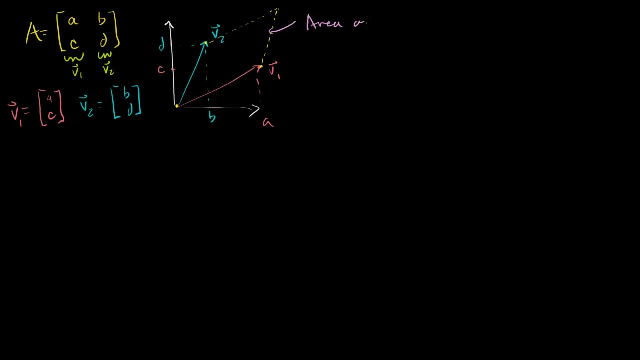 the area of the parallelogram generated by v1 and v2.. So how do we figure that out? So, in general, if I have just any parallelogram, this is kind of a tilted one. But if I just have any parallelogram, let me just 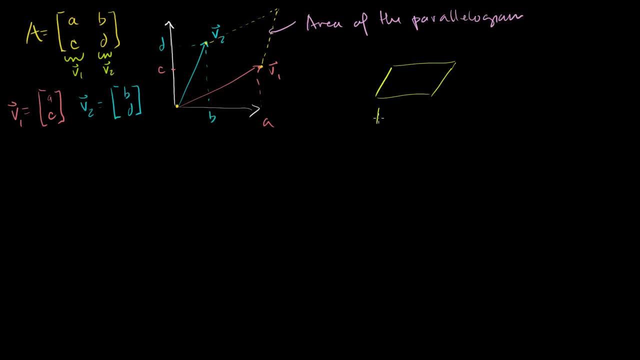 draw any parallelogram right there. The area is just equal to the base, So that could be the base times the height. So it's equal to base. I'll write capital B, since we have a lowercase b there. Base times height. 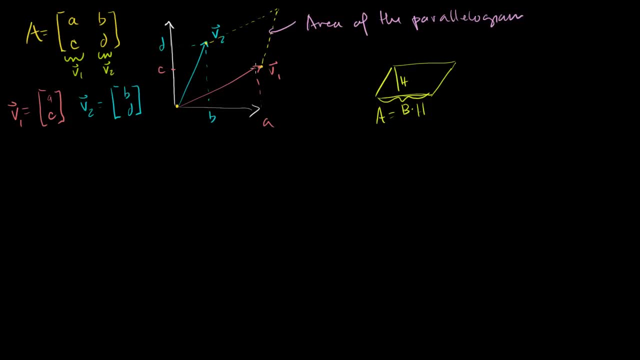 That's what the area of a parallelogram would be. Now, what are the base and the height in this situation? So let me write this down: The area of our parallelogram is equal to the base times the height, And actually, well, let me just write it here. 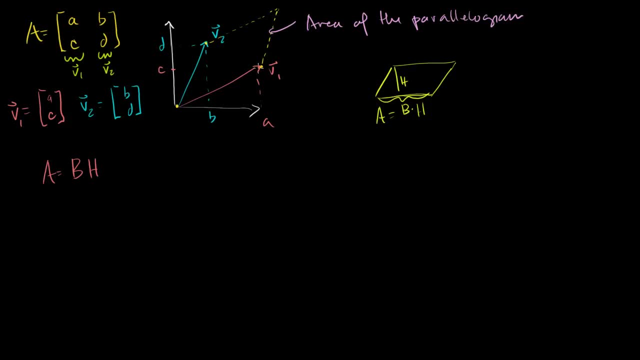 So what is the base here? The base here is going to be the length of our vector v. So this is our base. So this right here is going to be the length of vector v1.. The length of this orange vector right here. 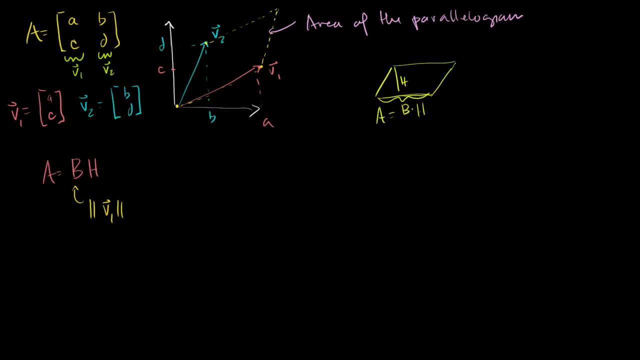 And what's the height of this parallelogram going to be? So we could drop a perpendicular here And the length of this line right here is going to be our height. So how can we figure out the? you know, we know what v1 is. 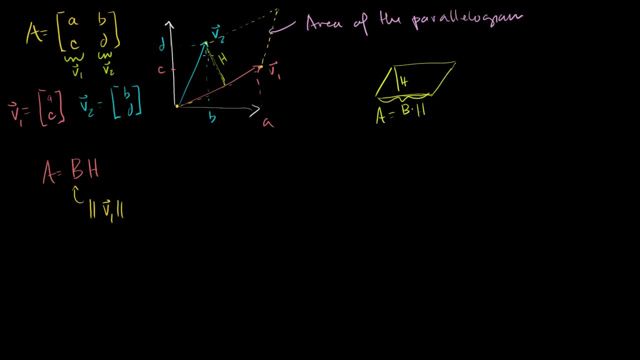 so we can figure out the base pretty easily, But how can we figure out the height? Well, one thing we can do is if we can figure out this guy right here. if we can figure out this guy, we could use a Pythagorean theorem. 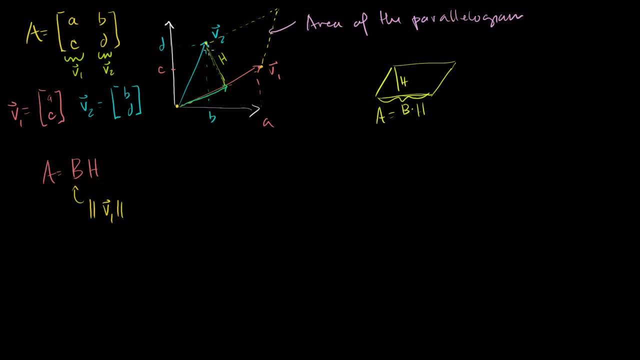 Because the length of this vector squared plus h squared is going to be equal to the length of v2 squared. So let's see if we can do that. What is this guy? What is this green guy right here? Well, if you imagine a line, let's imagine some line l. 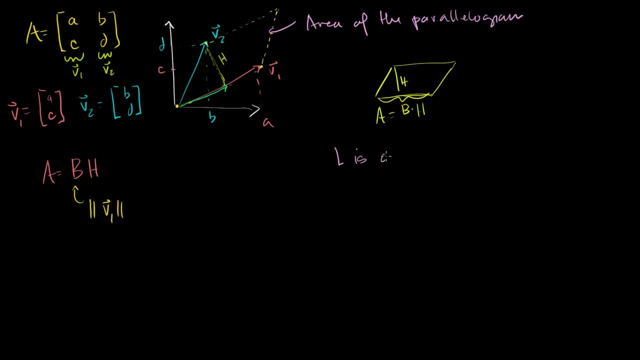 So let's say l is a line spanned by v1. Which means you take all of the multiples of v1, and all of the positions that they specify will create a set of points, and that is my line l. So you take all of the positions that they specify and that is my line l. 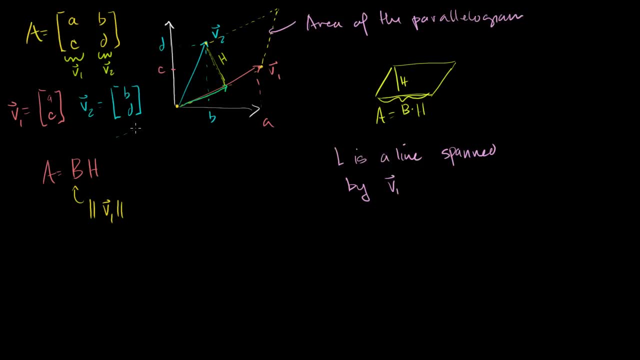 So you take all the multiples of v1, you're going to get every point along this line, Along a line that's like that. Now, if we have l defined that way, that line right there is l. and if you can see it, let me do it a little bit better. 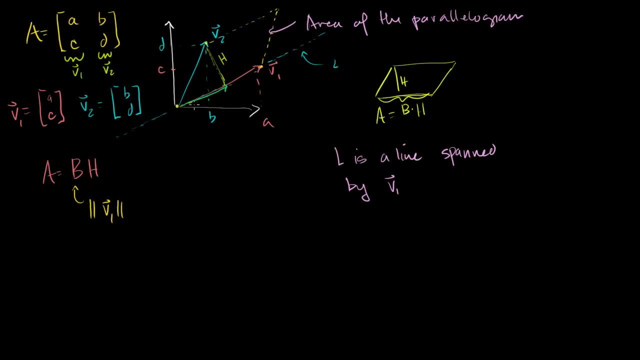 And it goes through v1 and just keeps going over there. What is this green line right there, This green line that we're concerned with? that's the projection. That is the projection onto l of what? Well, we have a perpendicular here. you could imagine a. 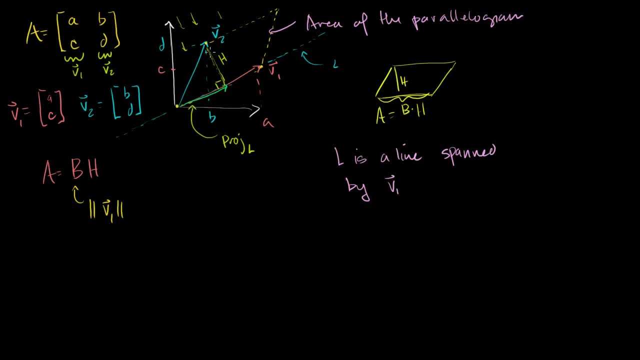 a light source coming down. I don't know if that analogy helps you, but it's kind of the shadow of v2 onto that line. So it's a projection of v2, of your vector v2 onto L. is this green line right there? 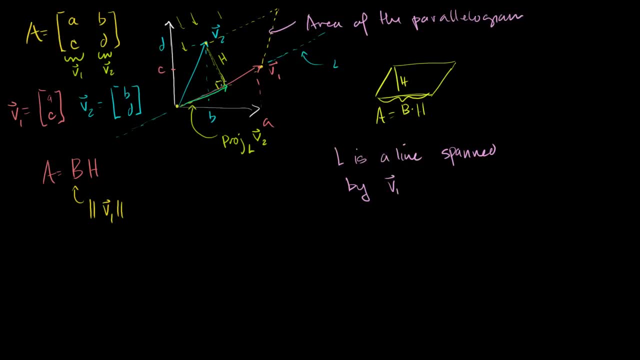 So if we want to figure out h, we can just use the Pythagorean theorem, So we can say that the length of h squared. or we could just write: well, I'm just writing h as the length, I'm not even specifying as a vector. 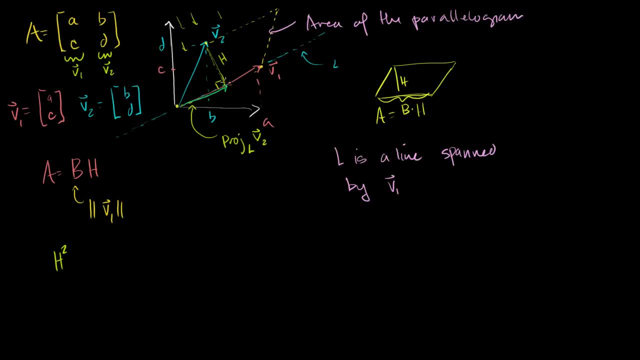 So we could say that h squared where that is the length of this line plus the length of this vector squared, and the length of that vector squared is the length of the projection onto L of v2.. I'll do that in a different color. 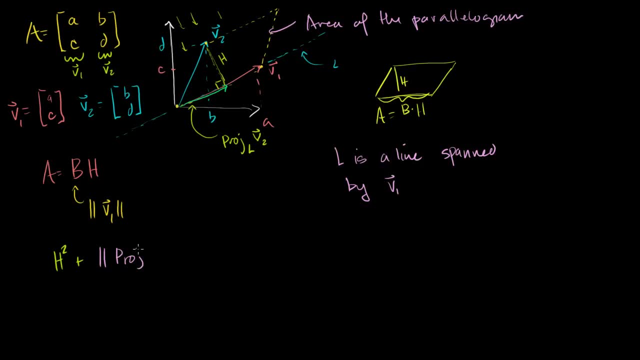 So the length of the projection onto L of v2 squared. we're just doing the Pythagorean theorem. This squared plus this squared is going to equal the length of this vector squared Equal that squared, It's going to be equal to the length of v2 squared. 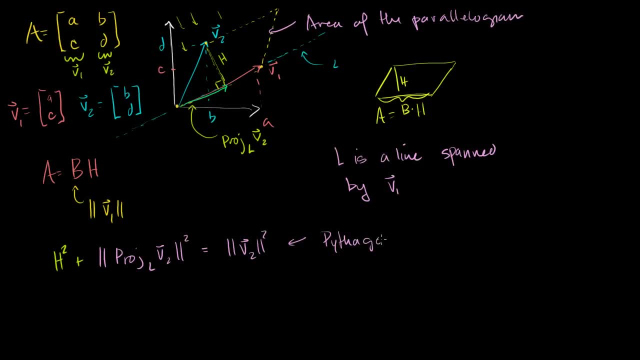 That's just Pythagorean theorem. Nothing fancy there. So how can we simplify? We want to figure out, we want to solve for h, And actually let's just solve for h squared for now, because it'll keep things a little bit simpler. 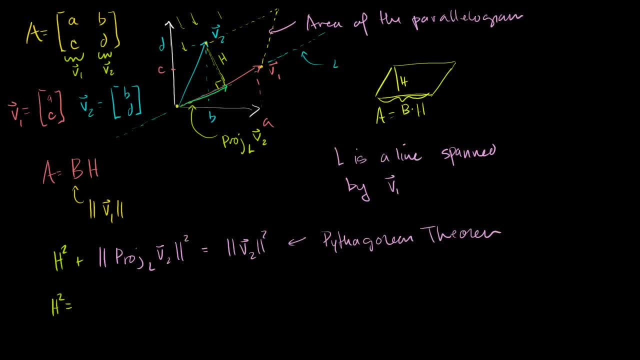 So we can say that h squared is equal to this guy. it's equal to the length of my vector, v2 squared, minus the length of the projection squared. So minus- I'll do that in purple- minus the length of the projection, the projection onto L of v2 squared. 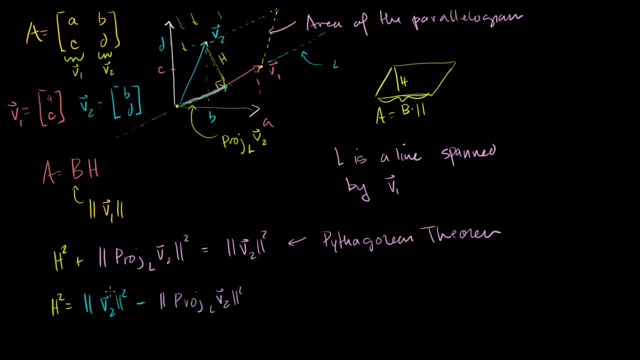 Remember, this thing is just this thing. right here We're just doing the Pythagorean theorem, So let's see if we can simplify this or write it in terms that we understand. So v2: squared: The length of a vector squared. 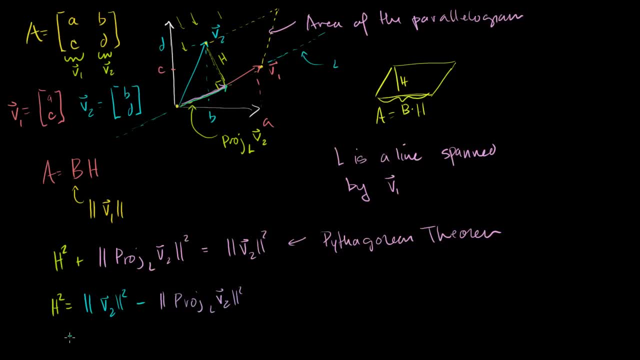 This is just equal to. let me write it this way: This is just equal to v2, dot, v2.. You take a vector, you dot it with itself and you get the length of that vector squared. We saw that many, many videos ago. 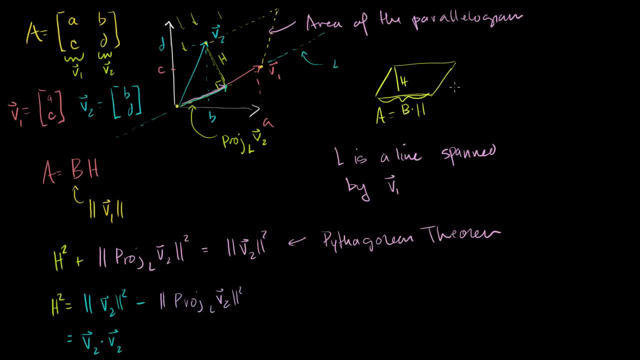 And then what is this guy going to be equal to? Well, the projection, I'll do it over here- The projection onto L of v2 is going to be equal to v2 dot, the spanning vector, Which is v2.. v1.. 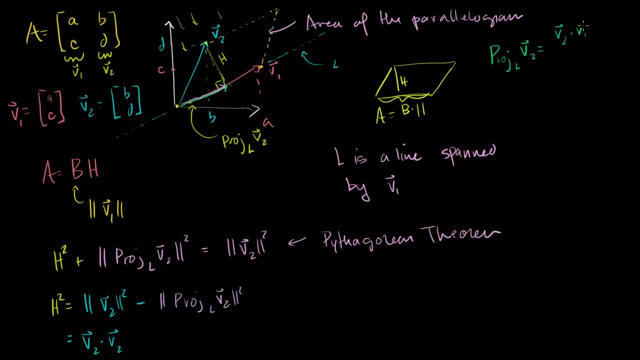 So it's v2, dot v1. over the spanning vector, dotted with itself: v1, dot v1.. We saw this several videos ago when we learned about projections. And this is just a number. This is just a number right there, And then it's going to be times, the. 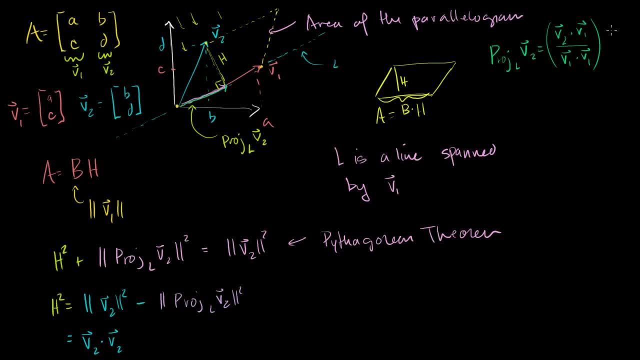 spanning vector itself. So times v1.. That is what the projection is. So it's going to be this: Minus the projection, the length of the projection squared. So what is the length of the projection squared? Well, that's this guy dotted with himself. 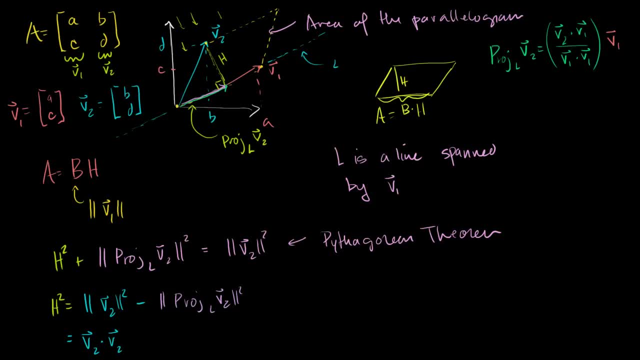 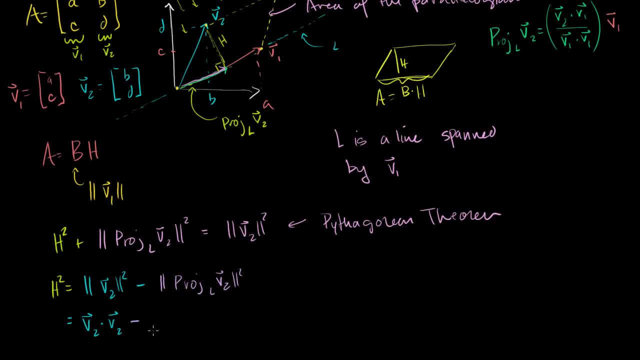 This guy dotted with himself. Let me write it this way. Let me take it step by step. So this is going to be minus. I want to make sure I can still see that up there so I don't have to write it. 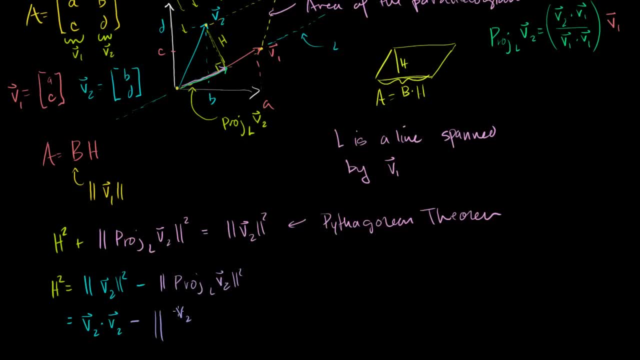 Minus the projection is going to be. it looks a little complicated but hopefully things will simplify. v2 dot. v1.. v1 over v1 dot. v1 times switch colors, times the vector. This is all just going to end up being a number. 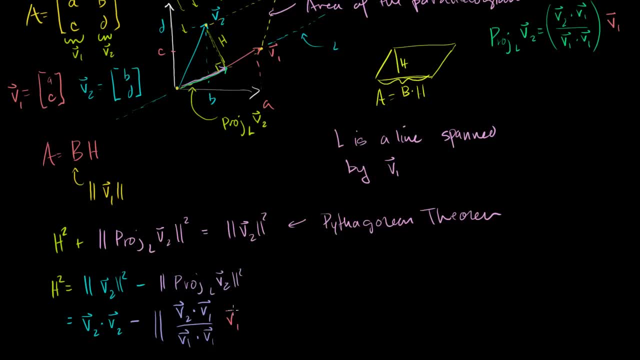 Remember, you take dot products, you get numbers, Times the vector v1.. And we're going to take the length of that whole thing squared And all of this is going to be equal to h squared. Once again, just the Pythagorean theorem. 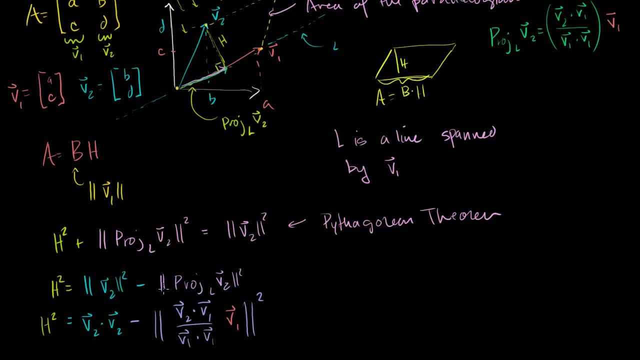 This squared, which is the height squared, Is equal to your hypotenuse squared. this is your hypotenuse squared, minus the other side squared. This is the other side squared. It looks a little complicated, but it's just the projection. 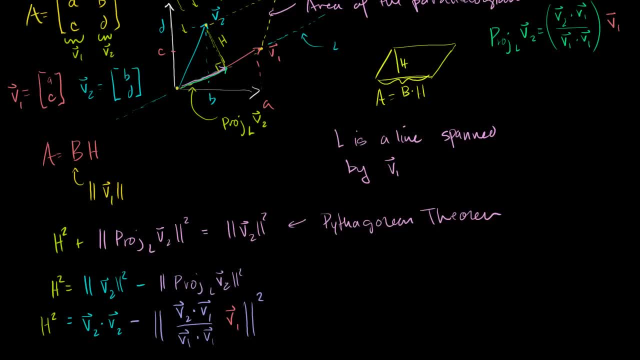 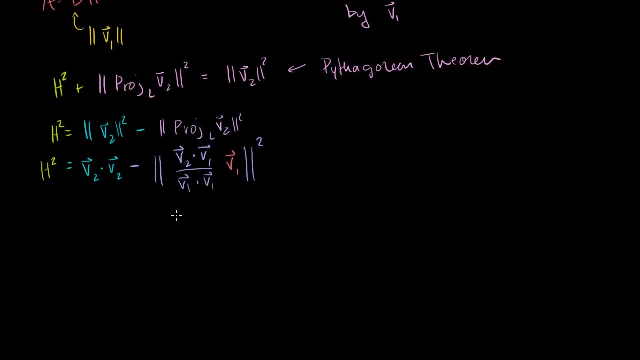 of this guy onto that right there. So let's see if we can simplify this a little bit. We're just going to have to break out some algebra, Or let's see what we can do here. Well, actually not algebra, some linear algebra. 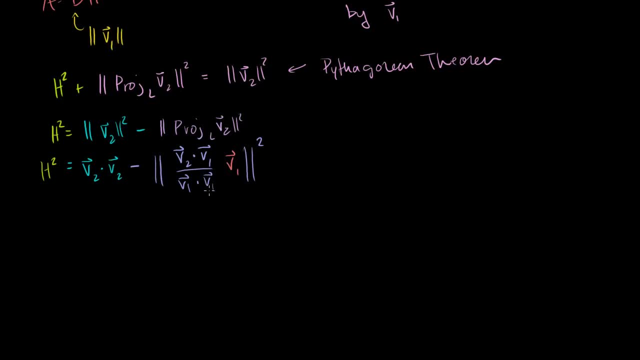 So what is this guy? Well, this guy is just the dot product of this with itself. So this is just equal to, We know I mean any vector if you take the square of its length. it's just that vector dotted with itself. 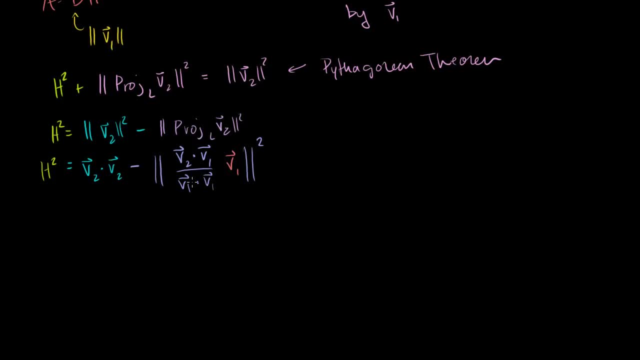 So this thing, if we take the square of this guy's length, it's just equal to this guy dotted with himself. So let me write everything over again, So we get h squared is equal to v2, dot, v2.. And then minus this guy dotted with himself, so minus v2, dot. 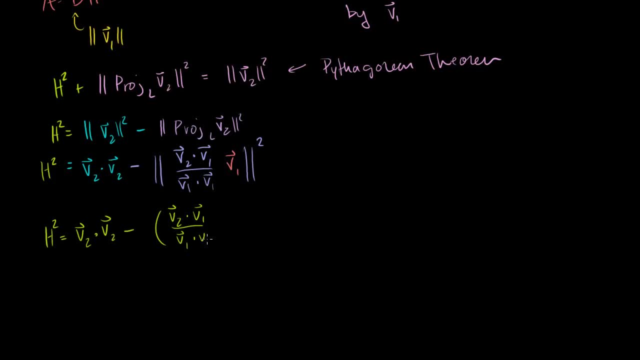 v1.. Over v1 dot v1 times the vector v1 dotted with itself. Dotted with v2, dot v1.. Remember, this green part is just a number. Over v1 dot v1 times v1.. And what is this equal to? 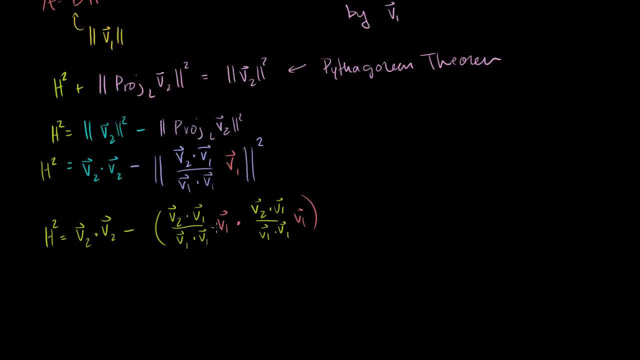 Let's just simplify this. These are just scalar quantities and we saw that the dot product is associated It is with respect to scalar quantities, So we can just change the order here. So this is going to be equal to the scalar quantity times itself. 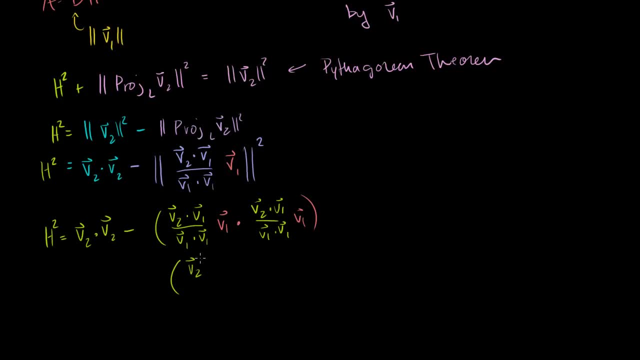 So, as we could say, this is equal to v2 dot v1.. Let me write it this way: v2 dot v1.. That's going to be, And then we're going to multiply the numerator times itself: v2 dot v1. 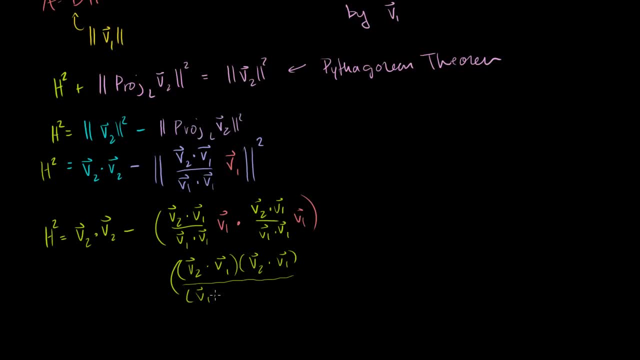 And then all of that over v1 dot v1 times v1, dotted with itself. v2 dot v1.. Remember, I'm just taking these two terms and multiplying them by each other. I'm just switching the order and then we know that the 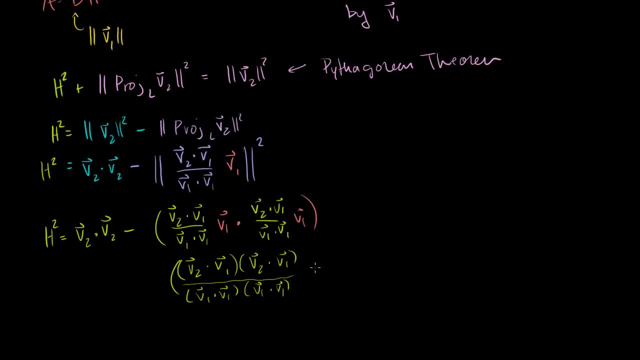 scalars can kind of be taken out. Times: these two guys dot each other. Times v1, dot v1.. That's what this simplifies to Now. this is now a number. We had vectors here, but when you take the dot product, you 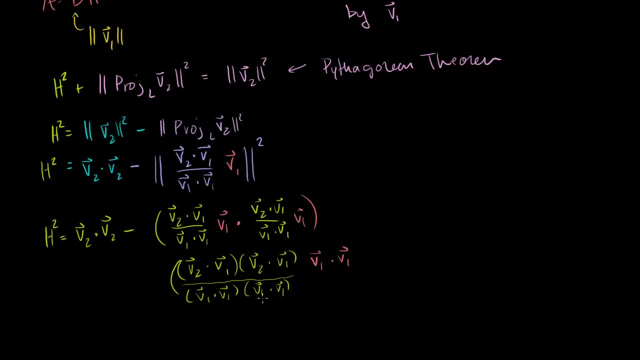 just get a number And this number is the same as this number. So we can simplify it a little bit, So we can cross those two guys out, And then we are left with that. our height squared is equal to this expression times itself. 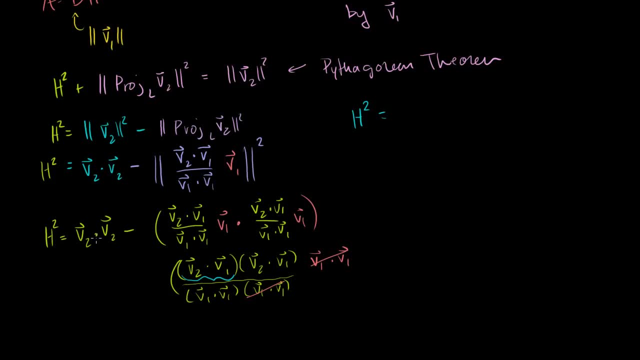 We have it times itself twice, So it's equal to. Well, let me start over here. It's equal to v2 dot- v2, minus this guy times itself. So v2 dot- v1. squared All of that over just one of these guys: v1 dot, v1.. 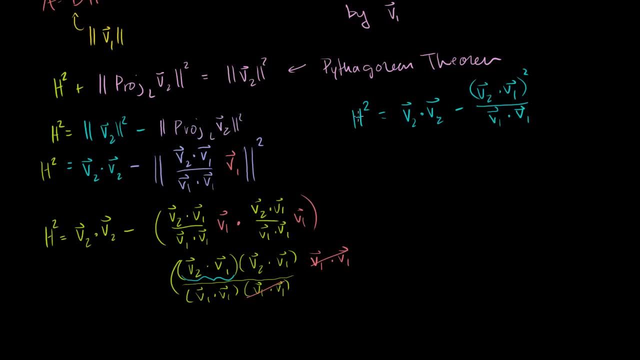 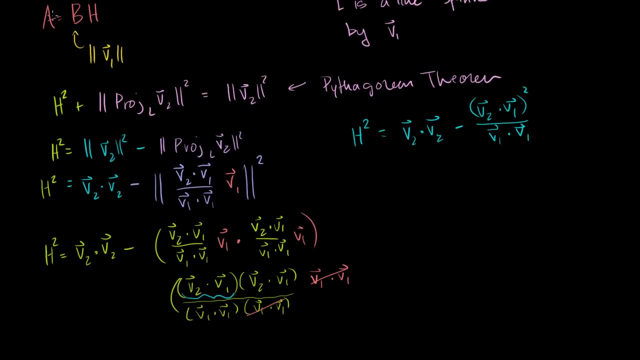 That is what the height squared is. Now we have the height squared. We could take the square root if we just want to solve for the height. but to keep our math simple, we know that area is equal to base times height. Let's just say what the area squared is equal to, because 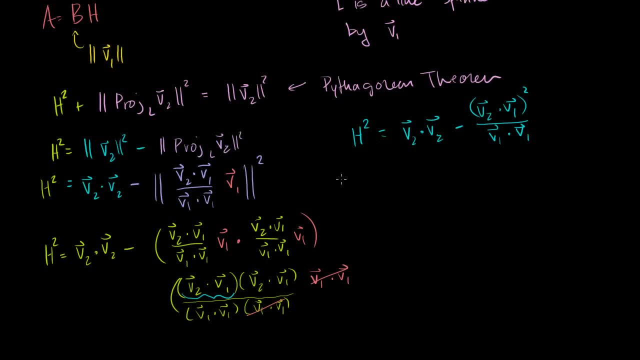 then both of these terms will get squared. So we know that the area is equal to base times height. We saw that at the beginning of the video. Then the area squared is going to be equal to these two guys squared. It's going to be equal to base squared, times height squared. 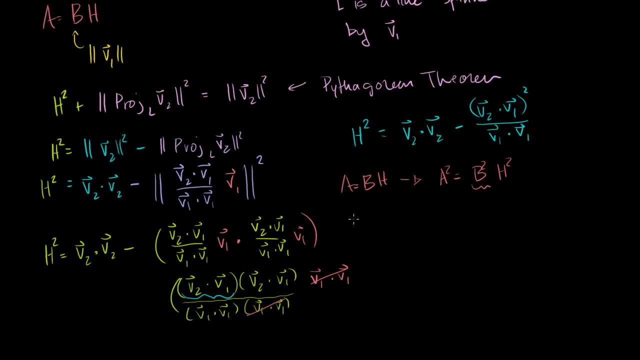 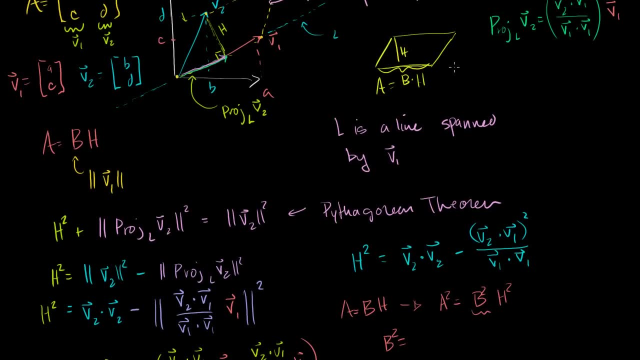 Now, what is the base squared? Let me do it like this: So the base squared- we already saw The base of our parallelogram- is the length, the base of our entire parallelogram. Remember, this is the parallelogram in question. 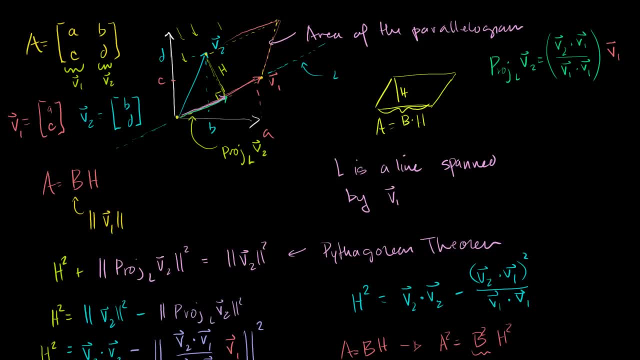 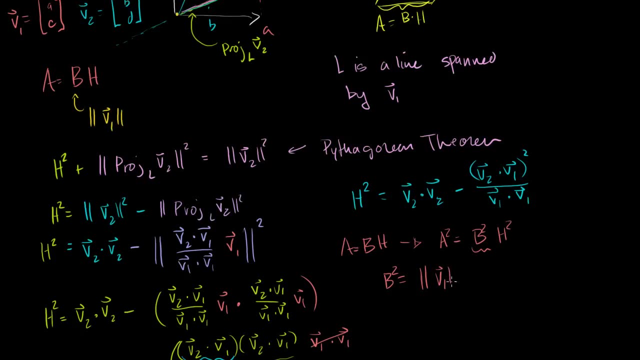 The base is the length of vector v1.. Now, what is the base squared? The base squared is going to be the length of vector v1 squared, or another way of writing that is v1 dot v1.. And we already know what the height squared is. 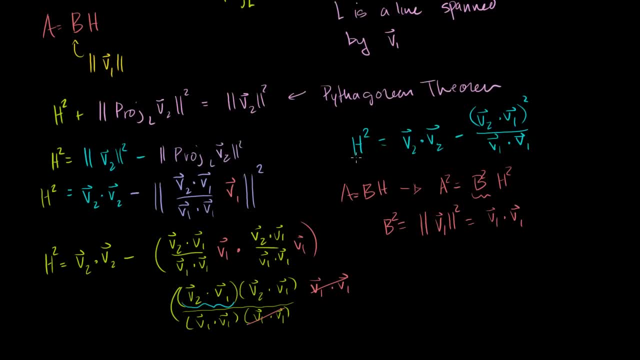 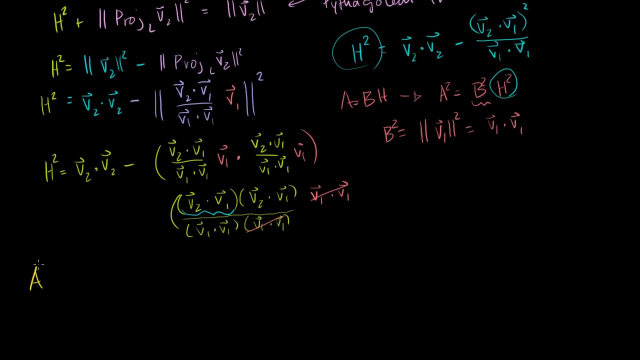 It's this expression right there. Let me write that down. The height squared is the height squared right there. So what is our area squared going to be? Our area squared- let me go down here while I have more space. Our area squared is going to be equal to our base squared. 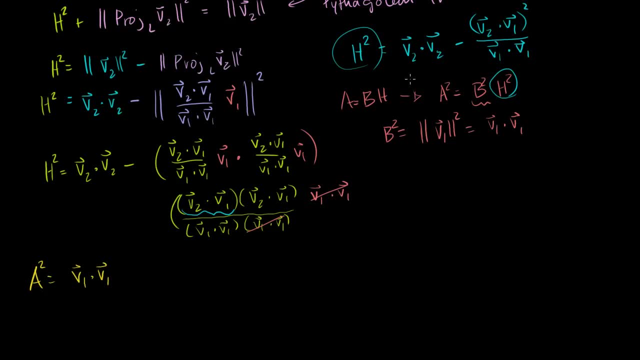 which is v1 dot v1 times our height, squared times this guy over here: v2 dot v2 minus v2 dot v1.. Now, what does this simplify to Well, this is just a number. These are all just numbers. 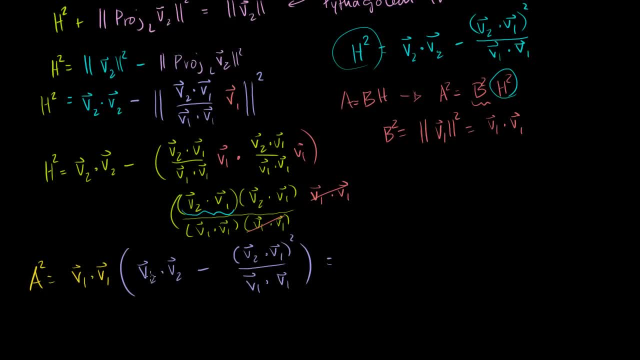 So if I multiply, if I distribute this out, this is equal to what? This times this is equal to v1,. let me write it color coded: v1- dot- v1 times this guy times v2 dot- v2.. And then when I multiply, this guy times that guy what? 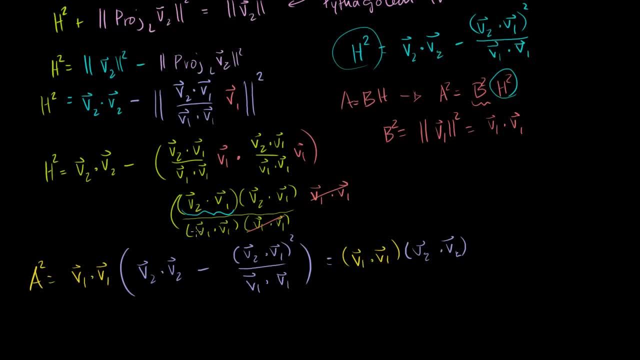 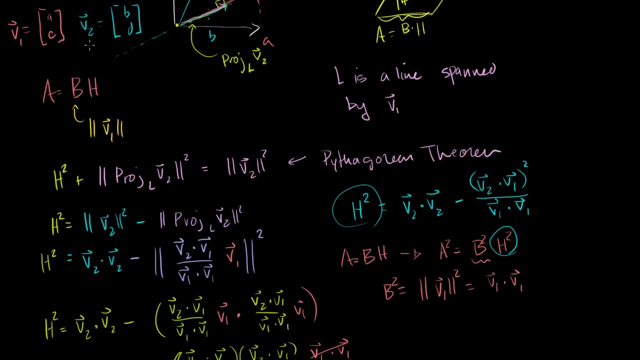 happens. Well, I have this guy in the numerator and that guy in the denominator, so they cancel out. So I'm just left with minus v2, dot v1 squared. Now let's remind ourselves what these two vectors were: v1 was the vector ac and v2 is the vector bd. 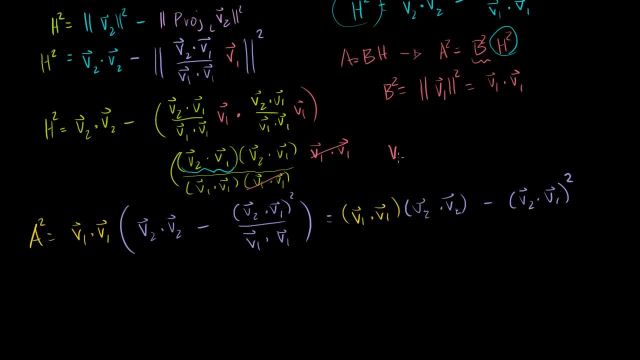 Let me rewrite it down here so we have it to work with. So v1 was equal to the vector ac And v2 is equal to the vector bd. So what is v1, dot v1?? That is equal to a dot a, which is or a times a, a. 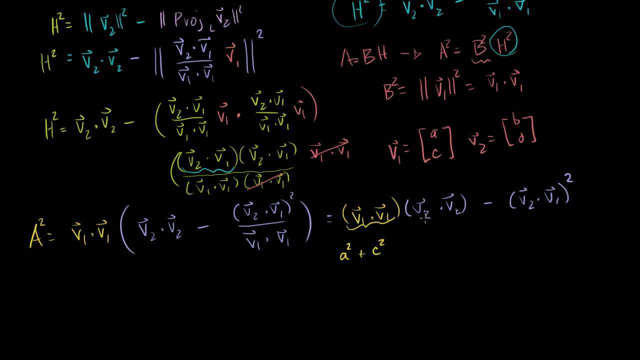 squared plus c squared. That's this right there, And that's what's: v2 dot- v2.. So we're going to have that times v2 dot, v2.. v2- dot- v2 is a v squared plus d squared. And then we're going to have minus v2 dot, v1 squared. 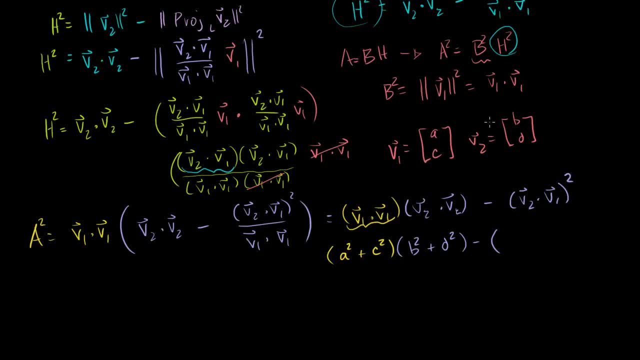 So what's v2 dot v1?? Well, it's b times a plus d times c, or a times b plus we're just dotting these two guys, so it's ab plus cd, And then we're squaring it. 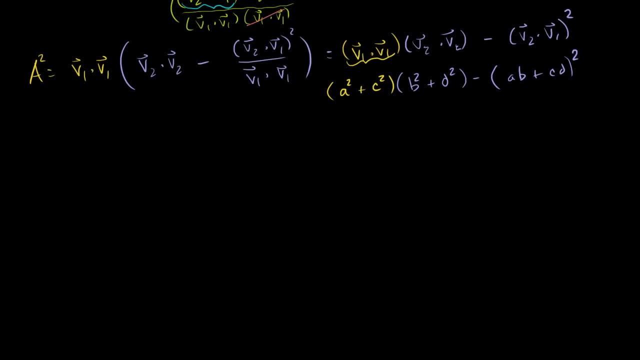 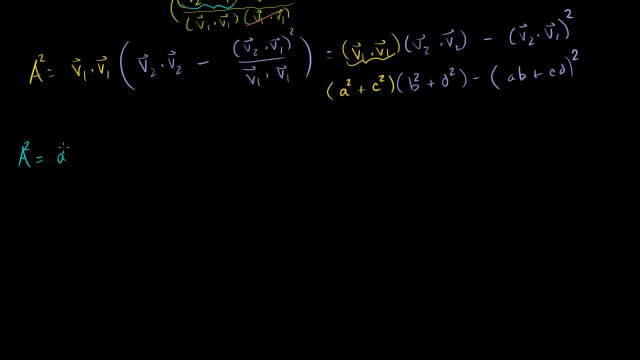 Our area squared is equal to a squared times b squared a squared b squared a. squared times d squared plus a. squared times d squared plus c. squared times b squared plus c. squared times b squared plus c squared times d squared. 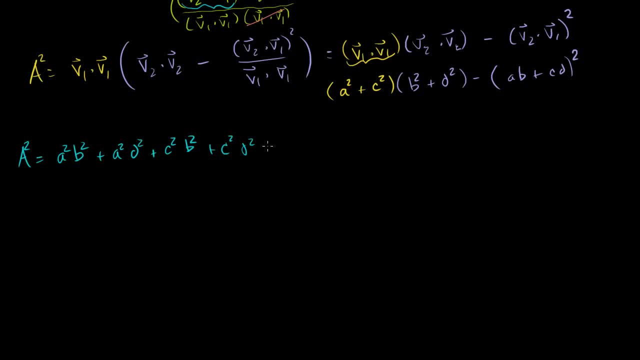 plus c squared, times d squared, and then minus this guy squared. What is that going to be equal to? ab squared is a squared, b squared, And then I have- I'm going to multiply these guys times each other twice, so it's going to be plus 2abcd, and then you're. 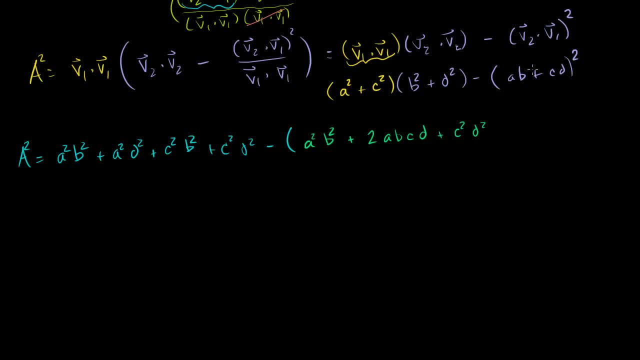 going to have a plus c squared d squared. I just foiled this out. That's the best way you could kind of think about it. And then, if I distribute this negative sign, what do I have? Let me rewrite everything. It's equal to a squared, b squared, c squared d squared. 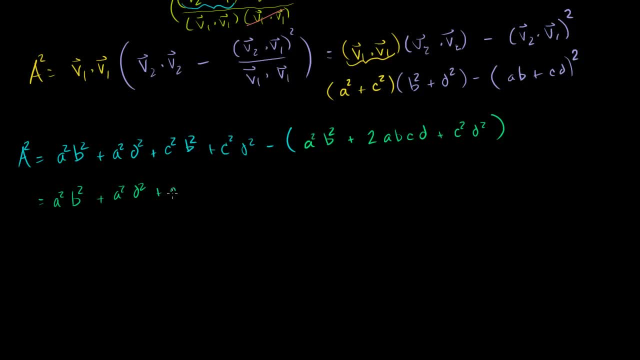 b squared plus a. squared d squared plus c. squared b squared plus c. squared d. squared minus a. squared b squared minus 2abcd minus c. squared d squared. All I did is I distributed the minus sign. Now it looks like some things will simplify nicely. 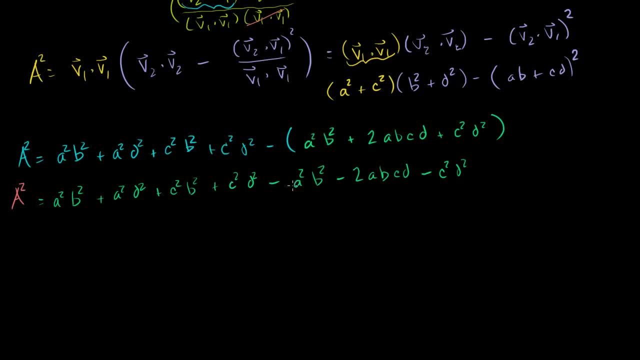 Remember, all of this was equal to our area squared. We have an ab squared. We have a minus ab squared. They cancel out. We have a minus cd squared and a cd squared, So they cancel out. So all we're left with is that the area of our parallelogram. 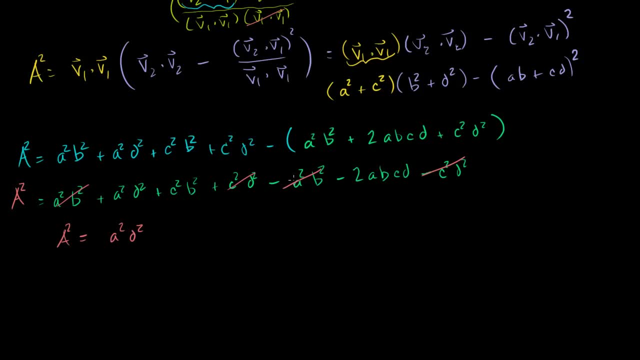 squared is equal to a squared, d squared minus 2abcd, plus c squared, b squared. Now this might look a little bit bizarre to you, But you might well. if you made a substitution right here, if you said that x is equal to ad and if you said y is equal to. 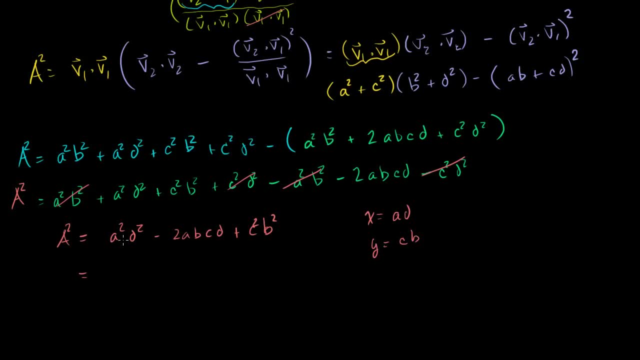 cb. then what does this become? This is equal to x squared minus 2 times xy plus y squared. Hopefully you recognize this. And this is just the same thing as x minus y squared. So what does this equal? It's 2y squared. 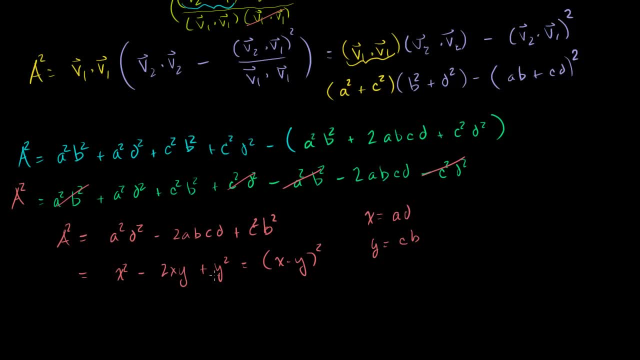 So this was our substitutions we made. I did this so you can visualize this a little bit better. So we have, our area squared is equal to x minus y squared, or ad minus cb, or let me write it: bc squared. That's what the area of our parallelogram squared is. 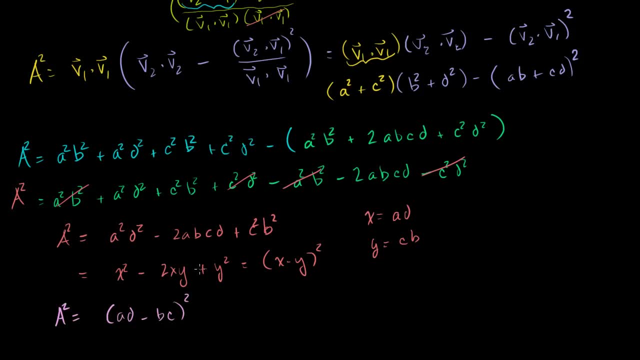 And if you don't quite understand what I did here, I just made these substitutions so you can recognize it better. but just to understand that this is the same thing as this: If you want, you can just multiply this guy out and you'll get that right there. 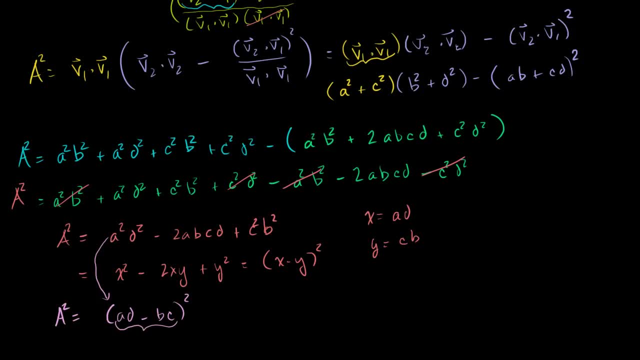 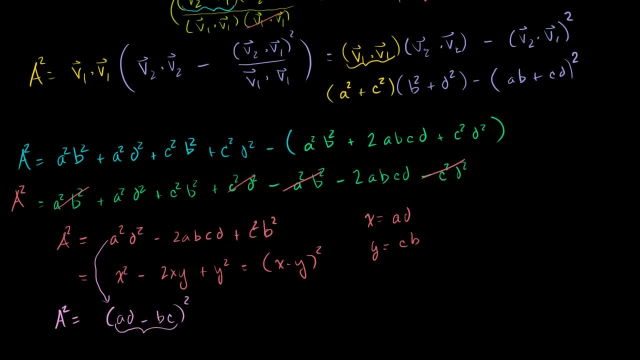 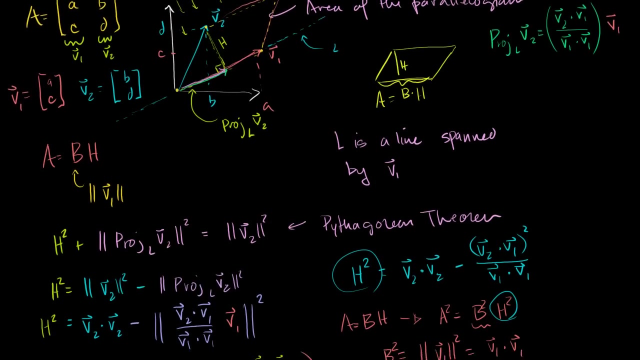 But what is this? What is this thing right here? It's the determinant. This is the determinant of our original matrix up here. Well, I called that matrix A, and then I used A again for area. so let me write it this way: 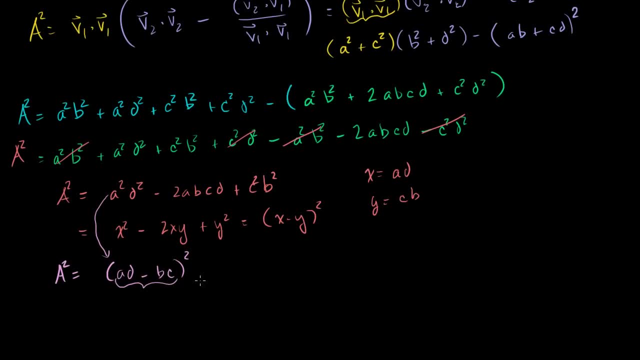 Area squared. Let me write it like this: Area, Area, Area squared. Area squared is equal to ad minus bc squared. So this is area. These A's are all area. But what is this? This is the determinant of my matrix. 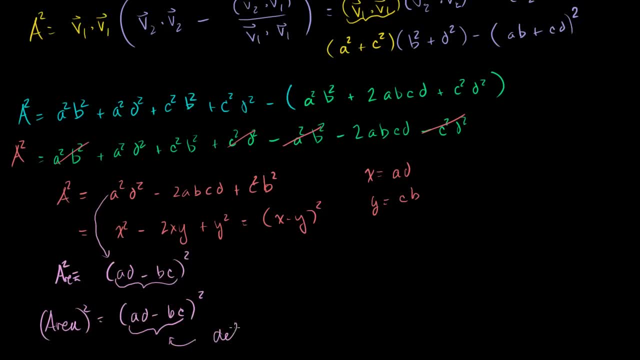 That is the determinant of my matrix A, my original matrix that I started the problem with, which is equal to the determinant of a, b, c, d. The determinant of this is ad. That is your core area, So I'm going to just divide that by B, B, b, c. 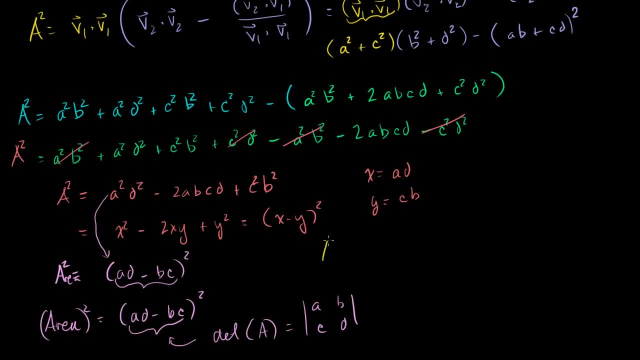 That's going to be the total area that I divide the average in. Well, what if B weren't here? What happens? What happens if it weren't here? Well, that's because the determinant of my matrix is going to wrap around me. 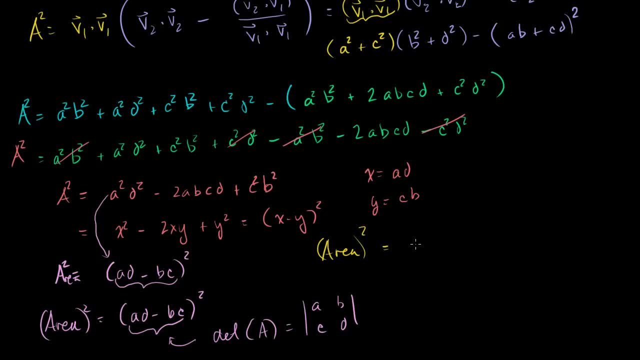 So I'm going to divide the error at the end of this sa and全部 and you can see that my matrix is: 일� kunt an Kop might not control that. The problem is that if you can divide it by the area, that's going to be alright. 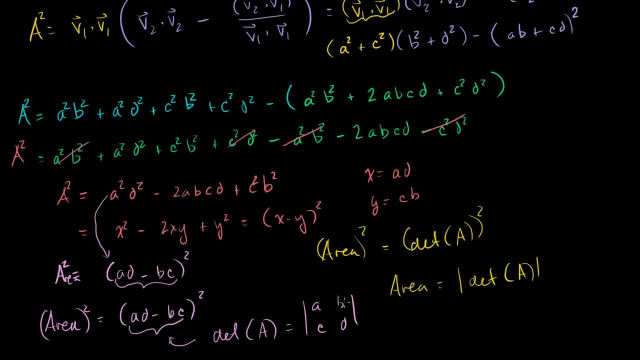 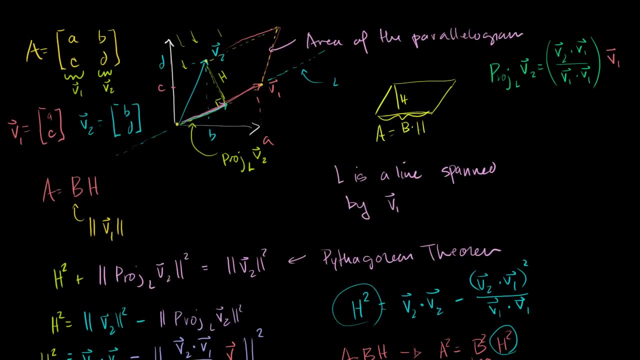 But you run the problem, You wind it up, Which is a pretty neat outcome, especially considering how much hairy algebra we had to go through. Let's go back all the way over here, Go back to the drawing. So if we want to figure out the area of this parallelogram, 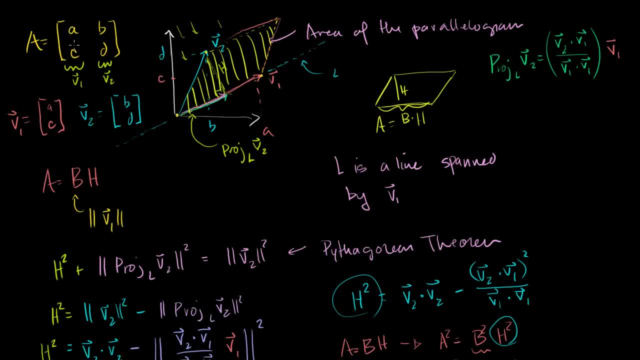 right here that is defined or that is created by the two column vectors of a matrix. we literally just have to find the determinant of the matrix. The area of this is equal to the absolute value of the determinant of A. And you have to do that because this might be negative. 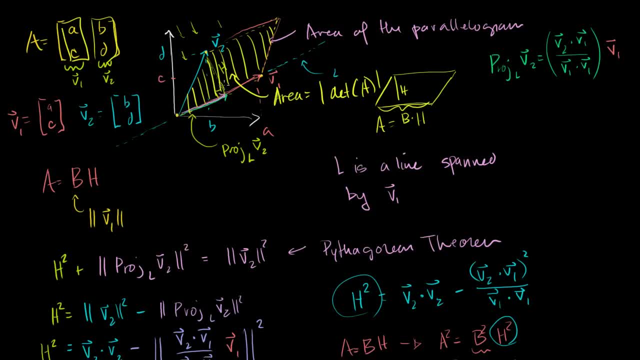 You could imagine if you kind of swapped these guys around, if you swapped some of the rows, this guy would be negative. but you can't have a negative area And it really wouldn't change what's spanned. If you switch v1 and v2, you're still spanning the same. 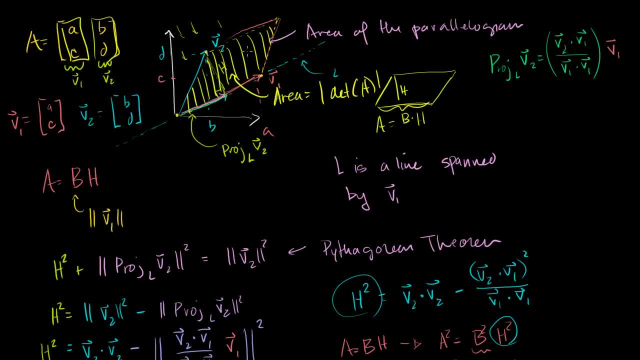 parallelogram, you just might get the negative of the determinant. But that is a really neat outcome And when you first learn determinants, you're going to have determinants in school. I mean, we learned the first motivation for a determinant. 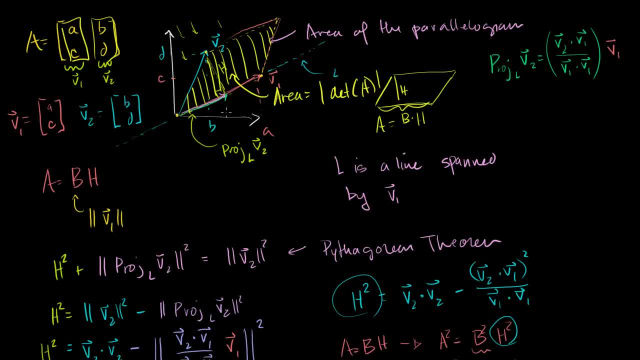 was this idea of. well, you know, when we take the inverse of a, 2 by 2, this thing shows up in the denominator. We call that the determinant. But now there's this other interpretation here, that it's actually the area of the parallelogram created by the. column vectors of this matrix.